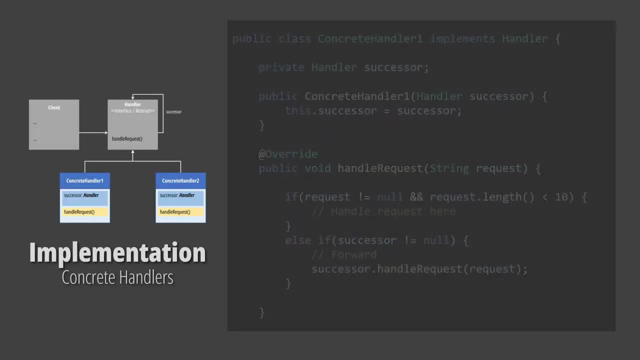 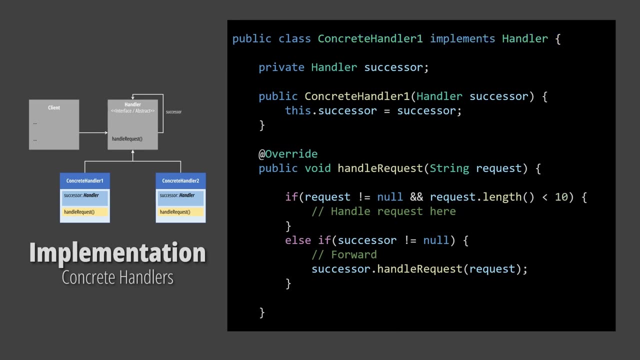 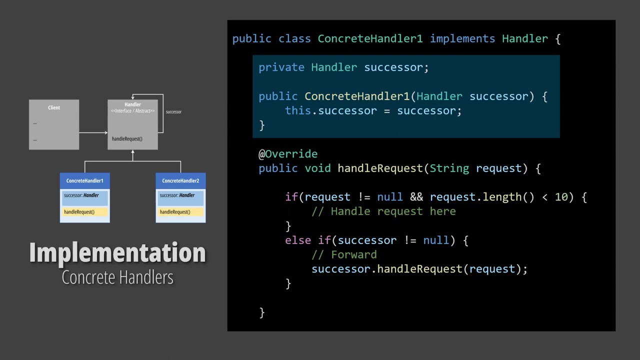 method. We then create concrete classes that implement the handler interface. These classes represent the links in our chain. There are two key concepts to notice. Each link has a reference to the next handler in the chain. In this example, we are setting the link right on. 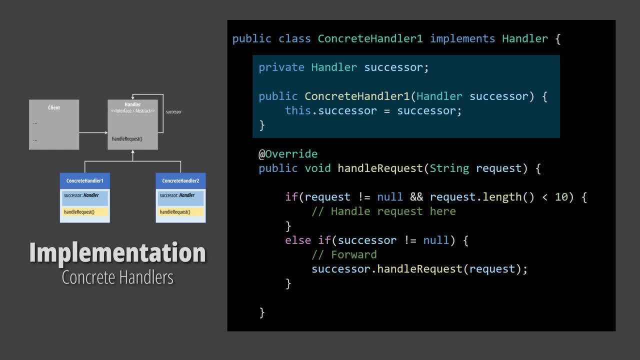 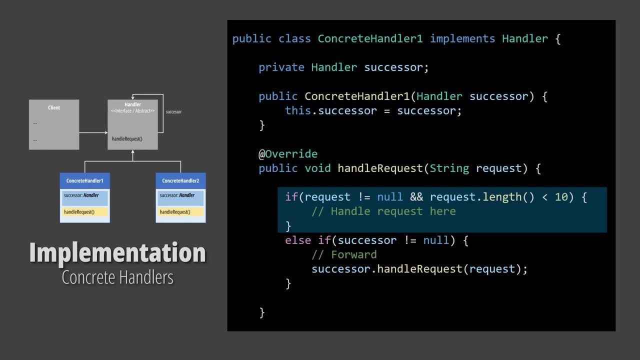 the constructor, but we could use setters instead. The other important concept is that each concrete handler has the ability to decide whether to process the request or forward it to the next handler. In this example, the concrete handler 1 handles the request only if it is less than 10 characters. 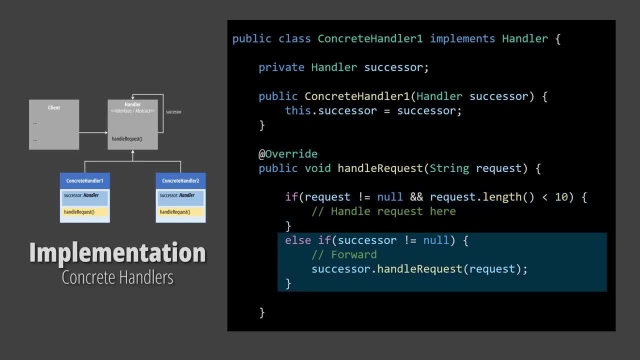 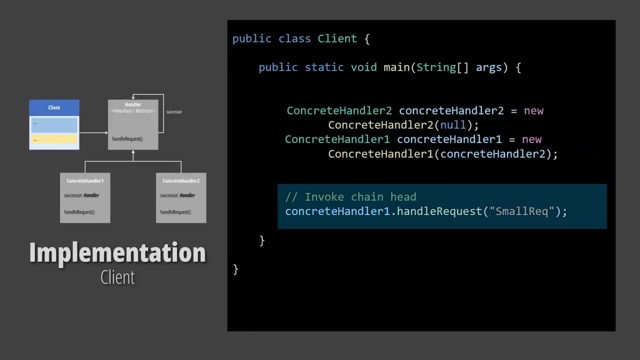 If it is larger, it forwards it to the next successor. This process continues until the request is handled or until there are no more handlers in the chain. Let's have a look at this example. The client's duty is to initiate the chain by invoking a handler, usually the first link. 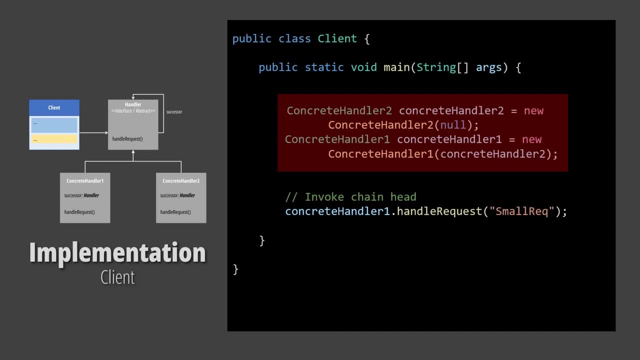 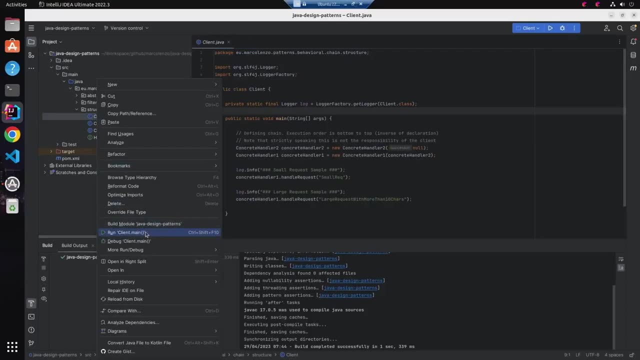 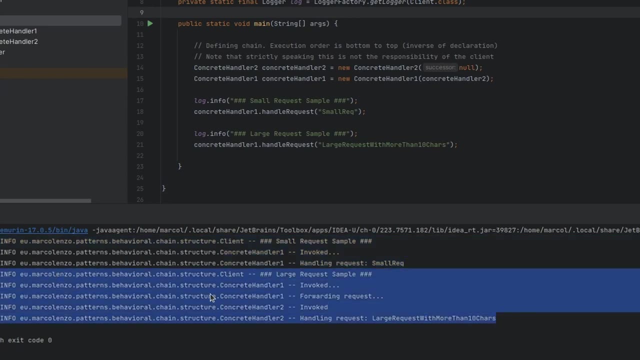 in the chain. In this code snippet, we are also setting up the chain in the same class. However, this is not the client's responsibility. If we look at the execution logs, the small request is handled by the first handler, while the larger request is forwarded on the second. 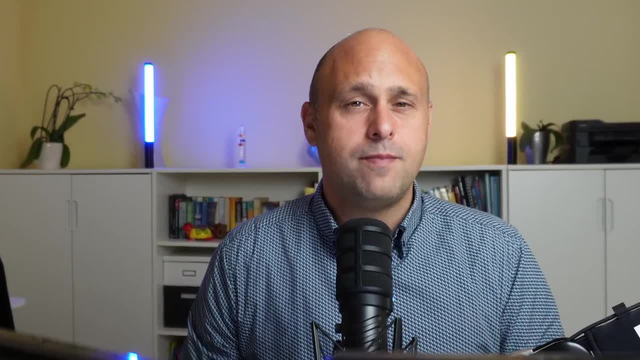 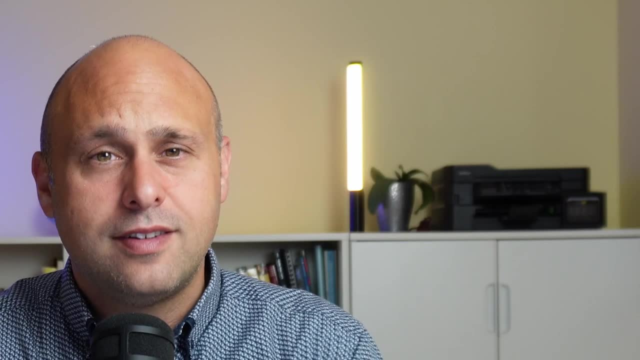 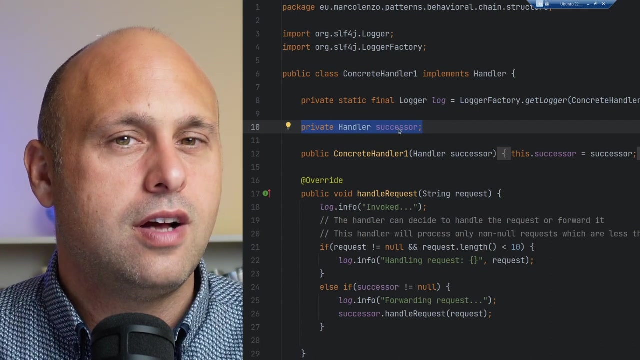 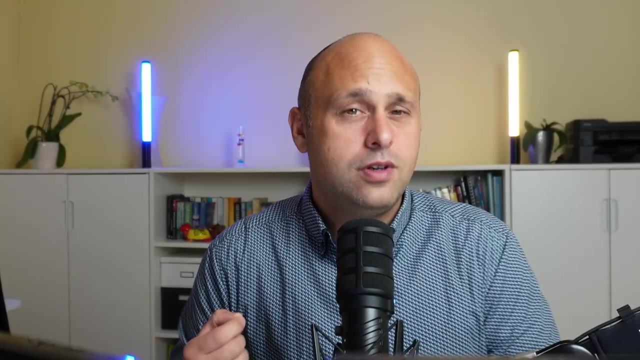 one. So what are the advantages of this pattern? The first one is that we have reduced coupling, Because the handlers have just the reference to the successor, but they invoke it through the interface. they don't need to know the target class, So there is not a direct dependency between an handler and another. For the very 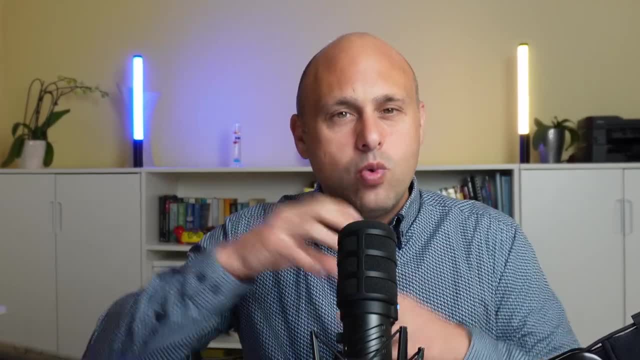 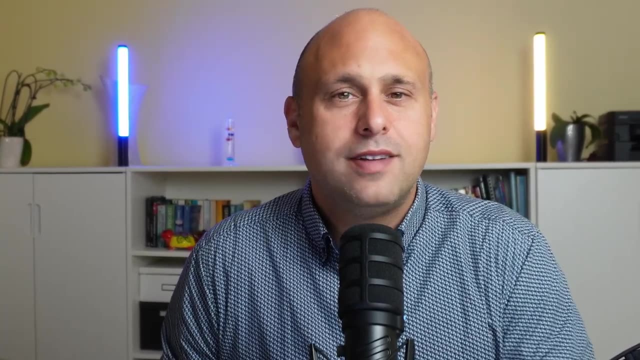 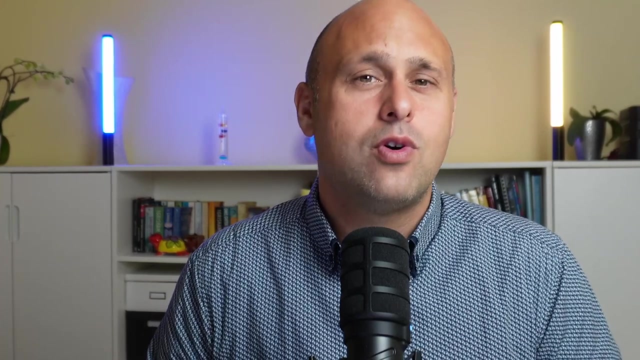 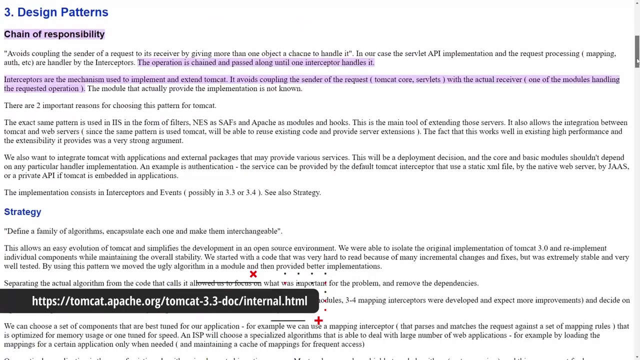 same reason. because there are no hard dependencies, we can swap the order of our handlers in the chain at runtime And we can basically modify the behavior of our application without having to rewrite any line of code in the handlers. A popular application of the chain of responsibility is the filter chain used to handle HTTP requests. 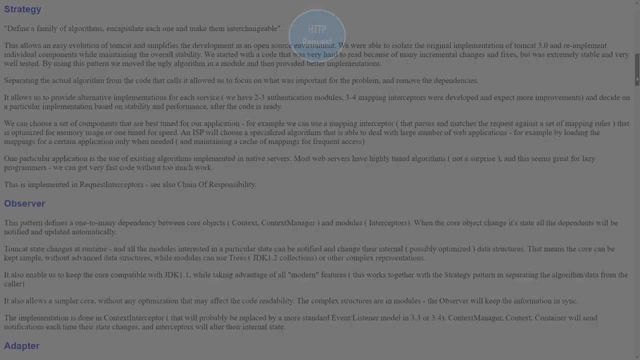 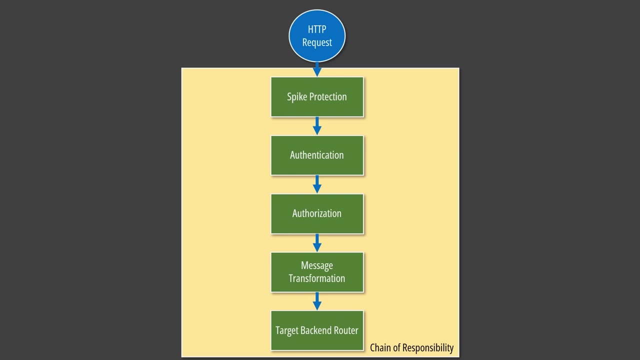 in a web server like Tomcat. You could use a similar approach to model an API gateway that processes a request and lets it pass it through policies, message transformers and a router. Keep in mind that this is not the case for any of the other applications. 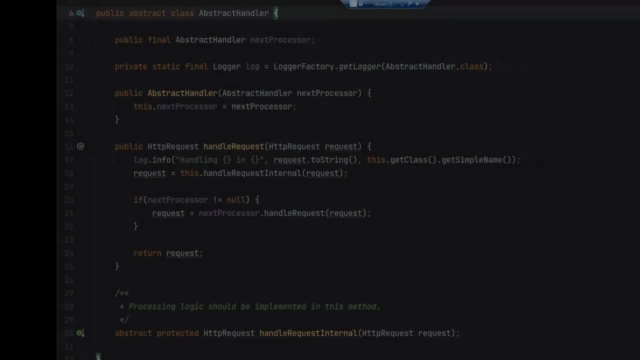 in the chain. You can also use a similar approach to model an API gateway that processes a request and lets it pass it through policies, message transformers and a router. Keep in mind that when dealing with these patterns, there are always variations In the chain of responsibility.